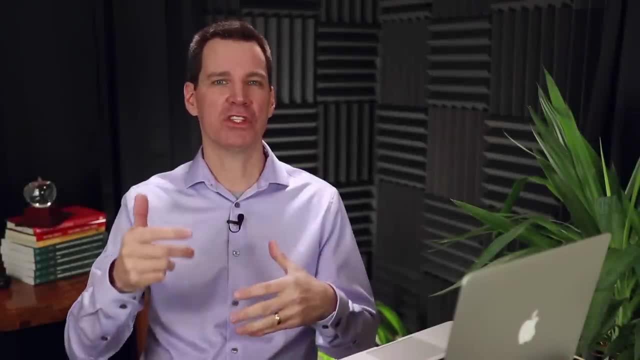 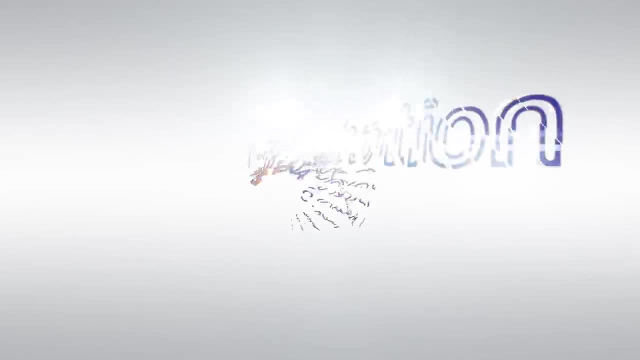 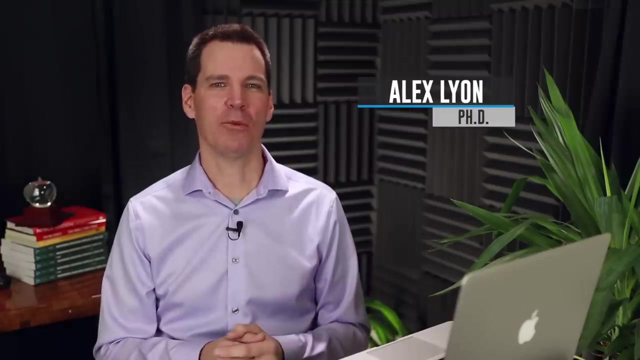 The way you practice a presentation directly influences the outcome. So in this video we're going to talk about how to practice a speech. Let's get into those details. Hello there, friends, Alex Lyon and we are at the end of a three-part series on public speaking. this 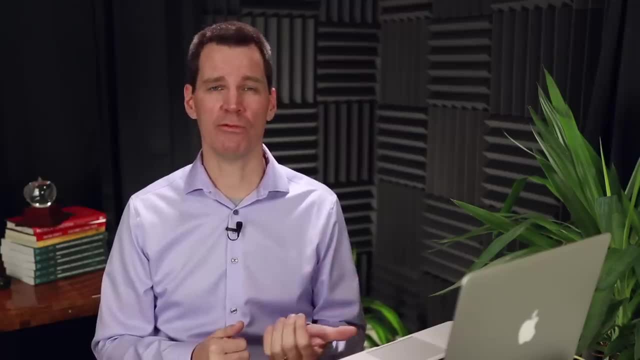 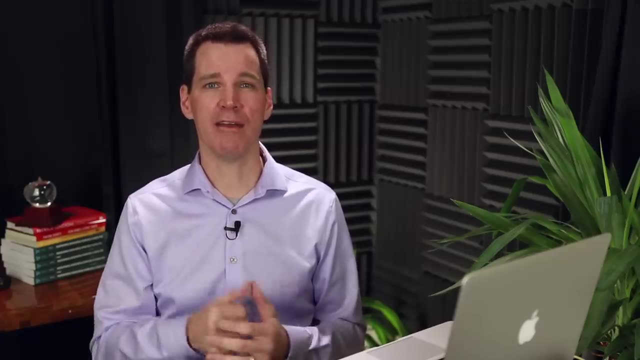 month. The first video is on the importance of public speaking, One before this is on how to improve and this one is specifically on how to practice a speech. So let's get into the five ways that I recommend you practicing a speech, And at the end of this video you may want to stick. 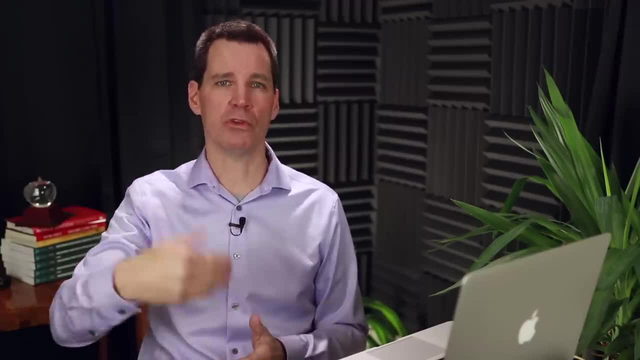 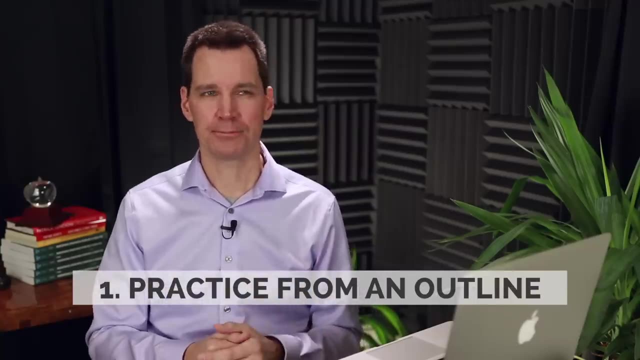 around, because I have a couple of resources to suggest to help you move your public speaking to the next level. So the first way to practice a speech is to practice from an outline, not word for word notes. I've given some version of this tip in a lot of different videos, but let's say: 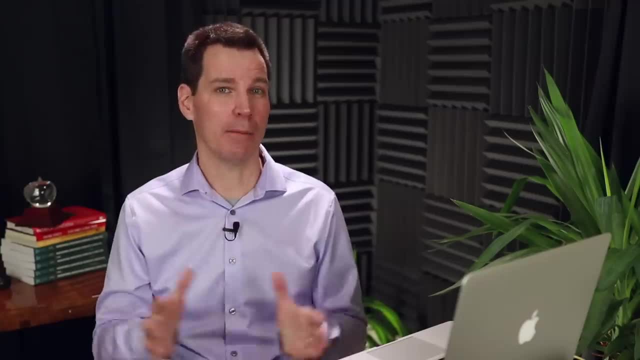 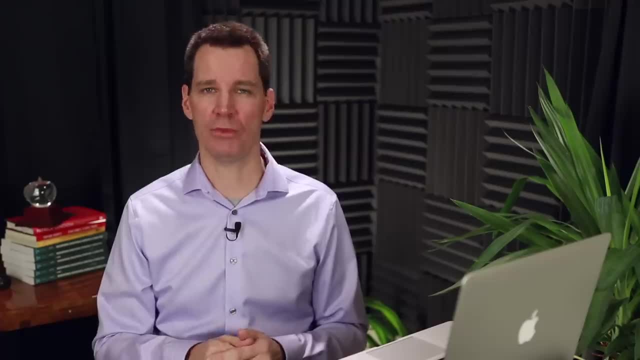 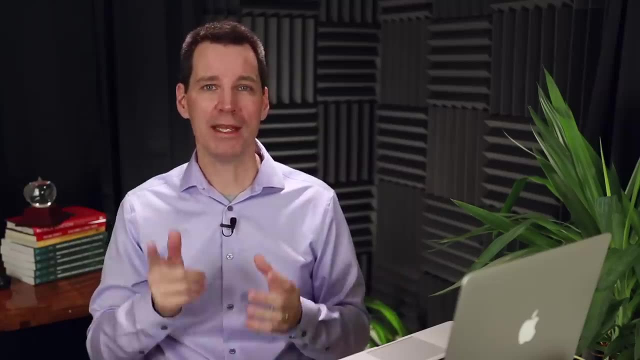 sound conversational, which is really what your listeners want from you. They don't want you to read your speech. They don't want you to sound like you've memorized it. They want a conversation, And the way to get there is this: You take whatever notes you have to prepare at first. 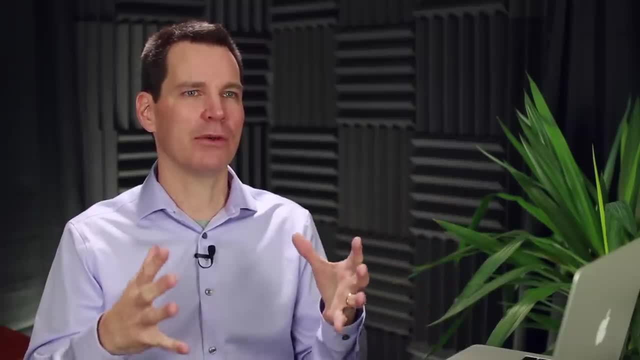 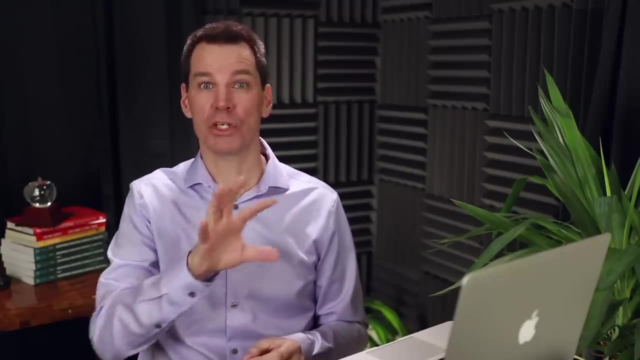 your first few drafts, and then you just keep cutting them down over and over again every time you practice, until all you're left with is a bulleted outline of your key points that you were going to hit. That's all you really want in the end, And that way you have a safety net. 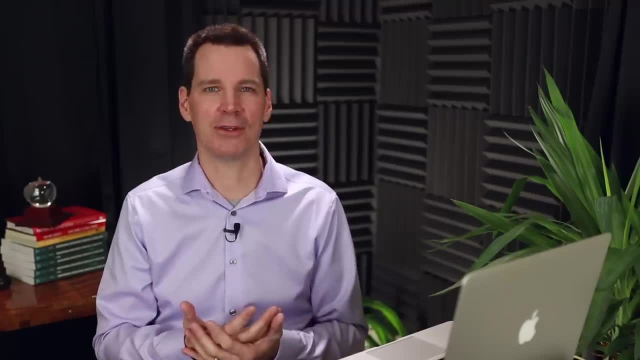 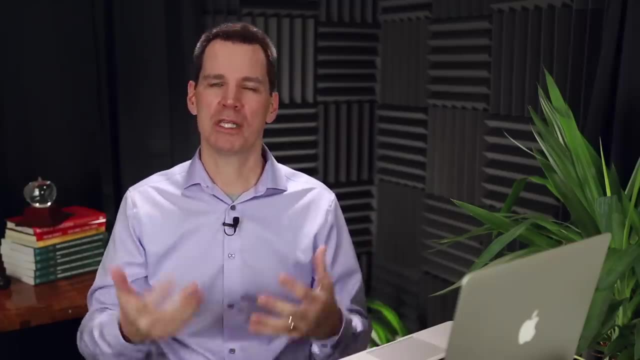 to fall back on so you won't ever lose your place. You can just glance down at your notes and then bounce your eyes right back up and present from an outline. That's the best way: Practice from an outline and, in the end, present like an outline. One of the things I will do, in fact, is: 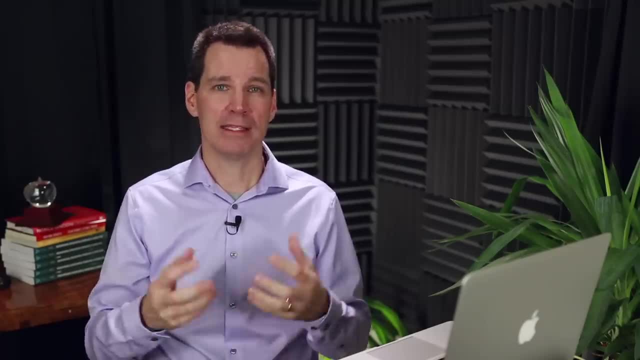 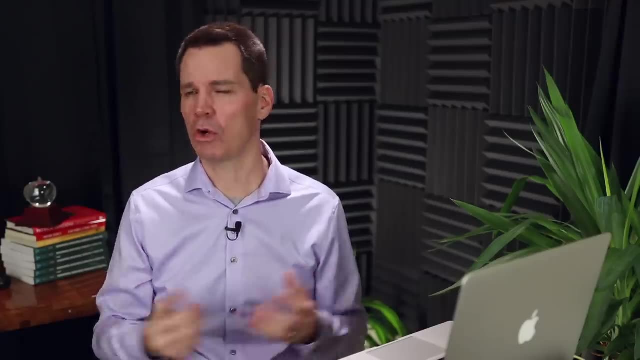 so I don't sound like I've memorized it. I don't sound like a robot is every time I practice. I might say it a little differently, on purpose, so that I'm not tempted to memorize. So don't try to put it word for word, Don't try to memorize talking points only, and practice from. 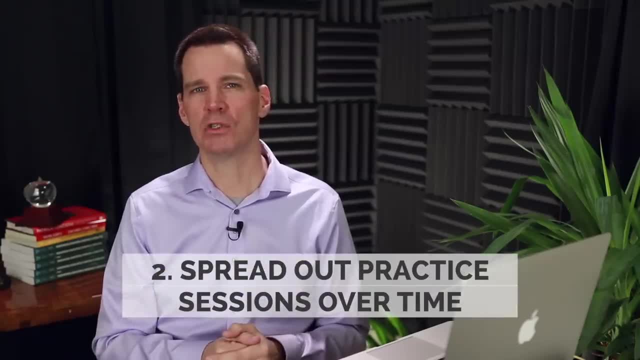 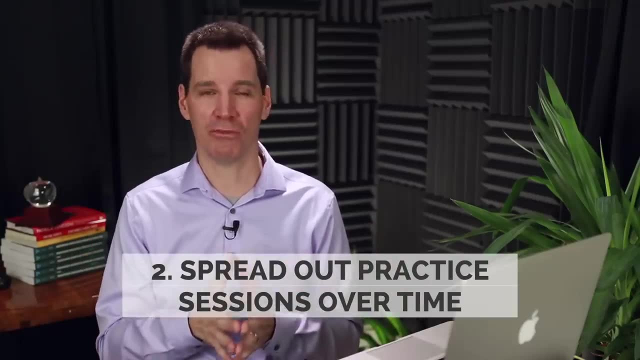 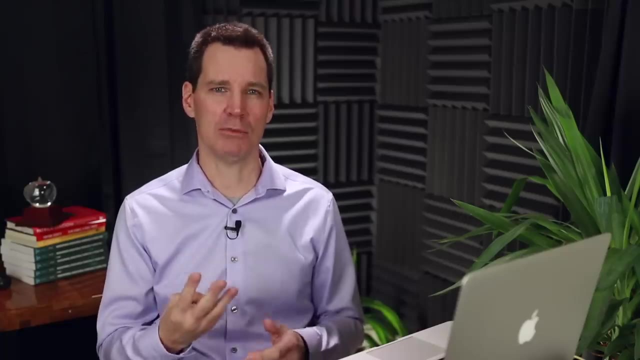 that kind of outline. The number two tip how to practice is to spread out your practice sessions over time. Don't cram the night before. Don't cram the morning before your presentation. I recommend spreading your practice sessions out over three days. The idea is to practice about three times. 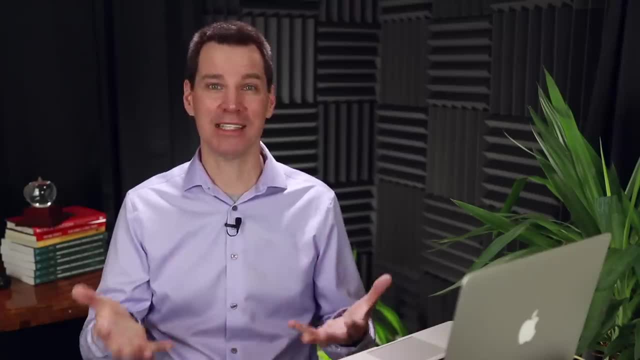 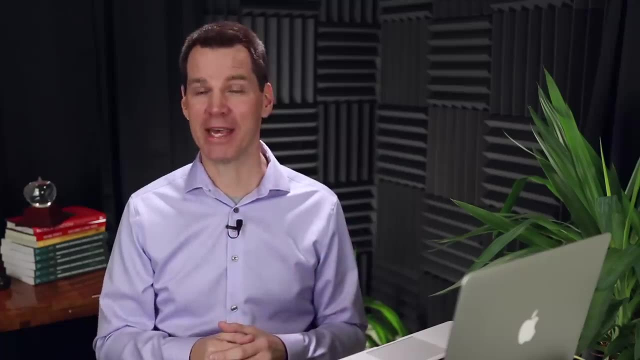 each day over those three days I like to practice about 10 times before I stand up and speak. and it's easier to do if you spread it out. A lot of great things happen when you spread out your practice sessions. The first thing that happens to me is it calms me down. It says to me: hey, there's time. 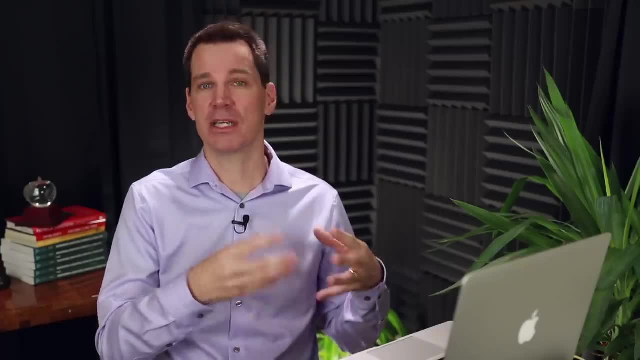 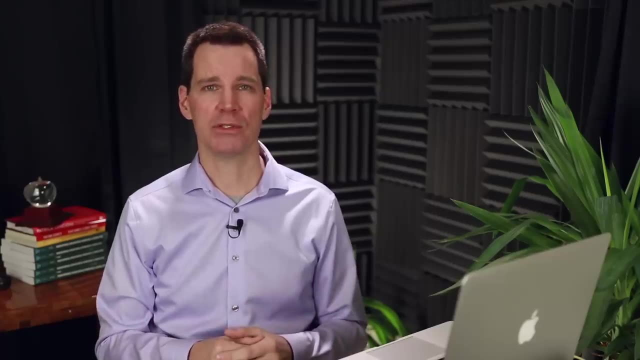 So if my earliest few practice sessions, practice times through, don't go so well, I say hey, there's time, No problem, I got a few more days, I'll work out these kinks. Another great thing that happens is, let's say, I practice it three times and then I sleep on it, Oftentimes in the middle of the day. 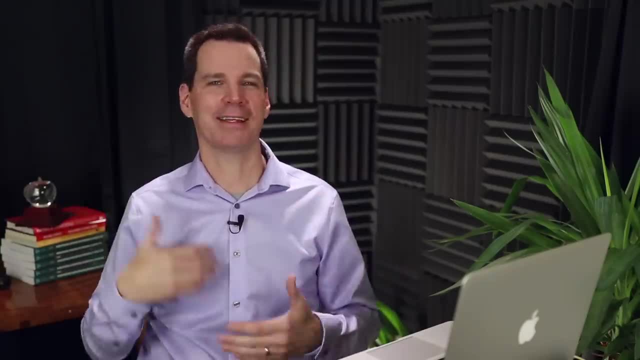 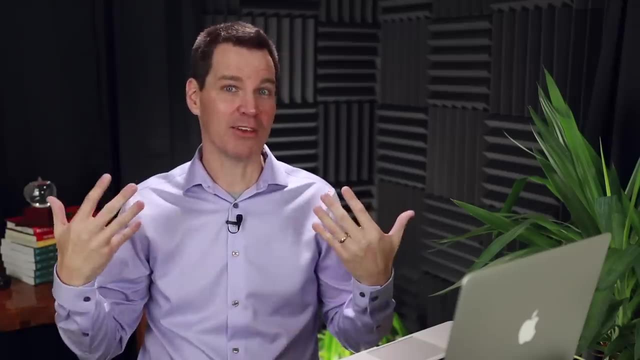 and I'm doing other things. I'm washing dishes, I'm working on it, and I'm working on it, and it keeps working on it and keeps figuring out better ways to say something or a quicker way to get to the point. So in that downtime, I believe, 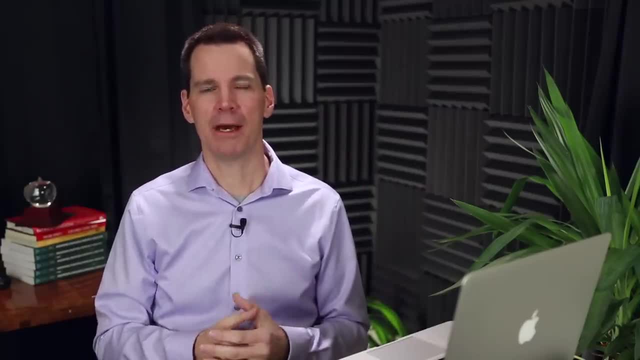 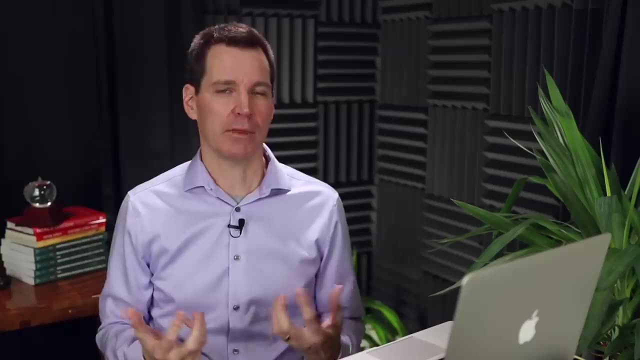 that our brains are still working on it and we benefit from that downtime as well. The other great thing about breaking up your practice sessions is it helps me with my composure in the moment, because it feels to me like muscle memory with an athlete that I've done this before. 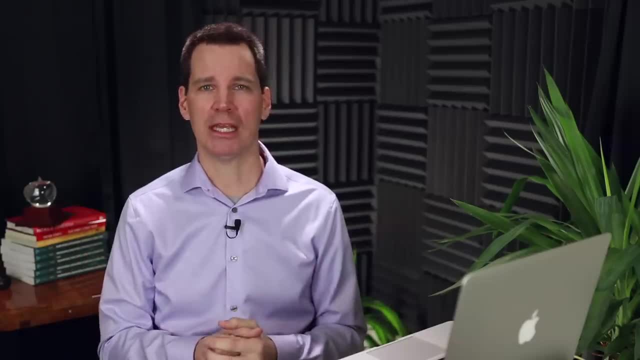 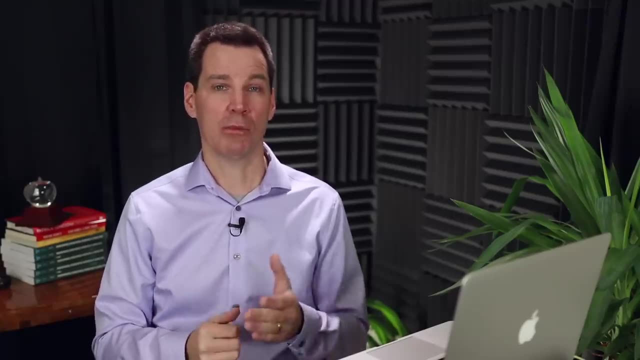 Like I've been doing this presentation for days, So it really helps me stay composed. so spread out those practice sessions three times a day over three days. That usually is about what you need. The number three tip is to focus on only one or two improvements each time you practice it. 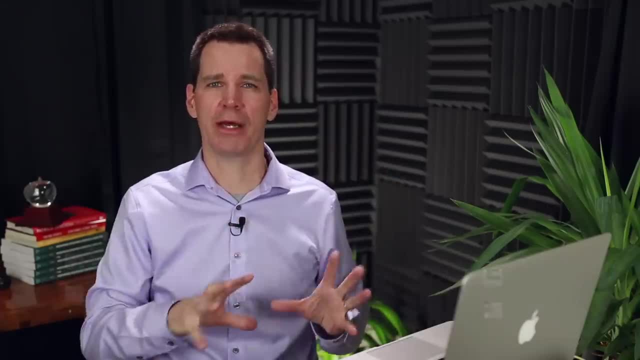 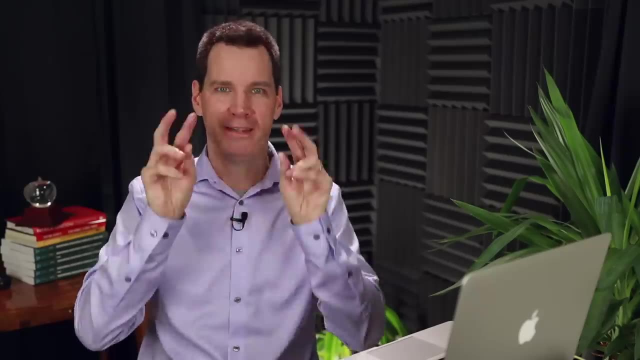 through. So you might just work on your structure and your outline the first few times through, That's normal. The next few times through, just pick one or two things like: oh, now I'm just going to work on looking up from my online eye contact, for example, The next. 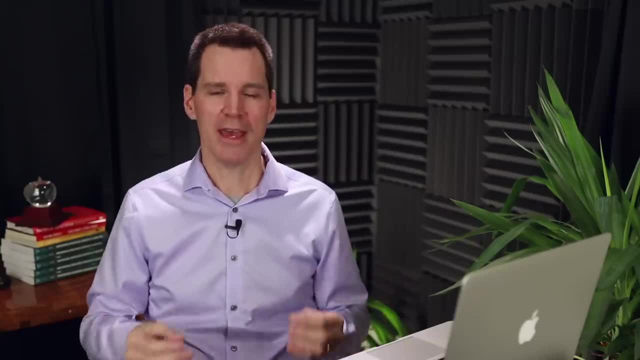 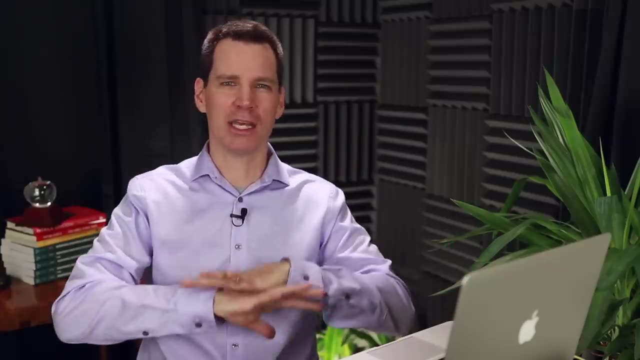 time through. you might just work on gestures and your posture a little bit. Every time you practice, add one or two things you want to improve on, because when you add too many things all at once, when you try to get it perfect every time you practice, you're going to get paralyzed because 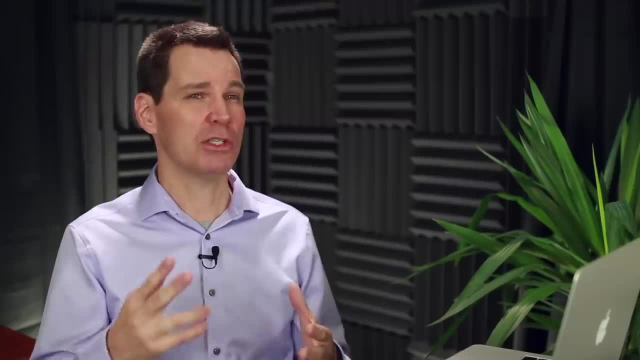 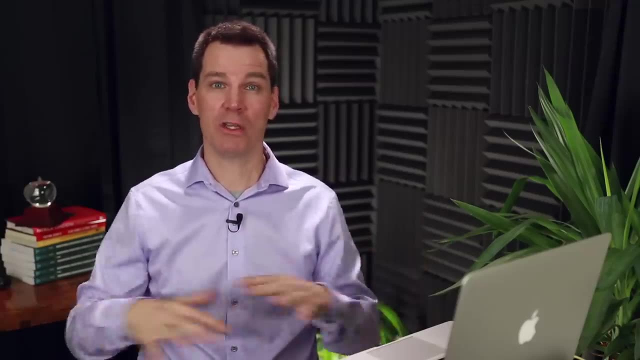 you can't really improve more than one thing, or maybe two things, in any given practice session. So focus on improvements and then start checking those off the list, And then your fundamentals will all be in place by the time you actually stand up to present. Number four tip is to keep. 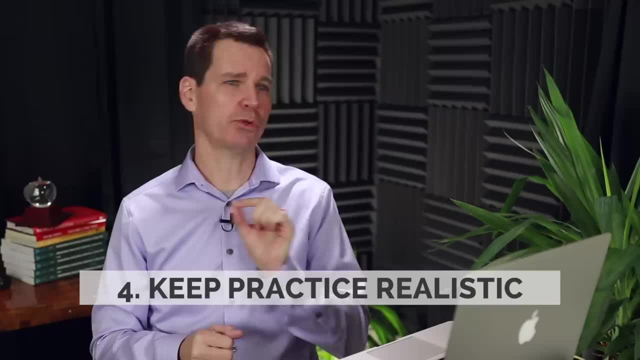 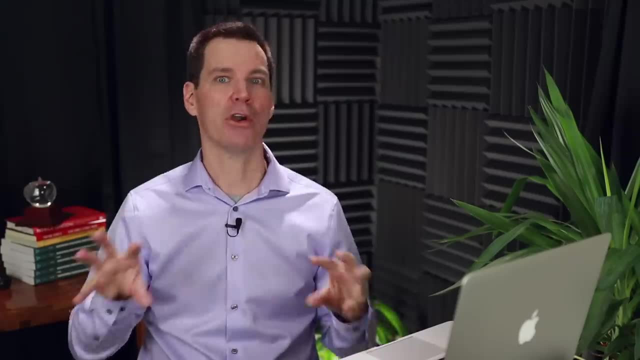 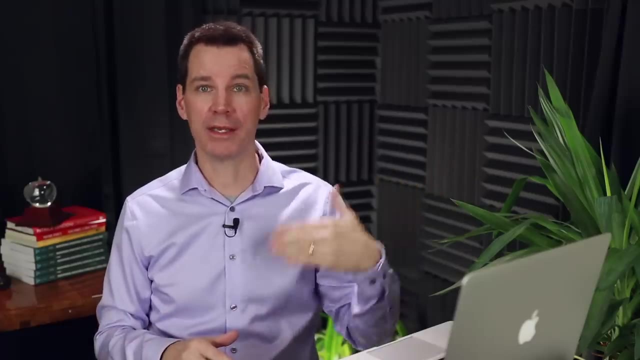 practice sessions realistic. Do not, for example, the whole time you're practicing, isolate yourself completely and make conditions perfect, because what ends up happening in the moment of your actual presentation is: it won't go perfectly, People will walk in late or they'll. 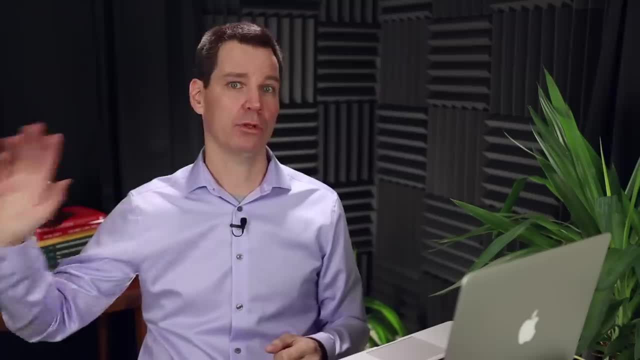 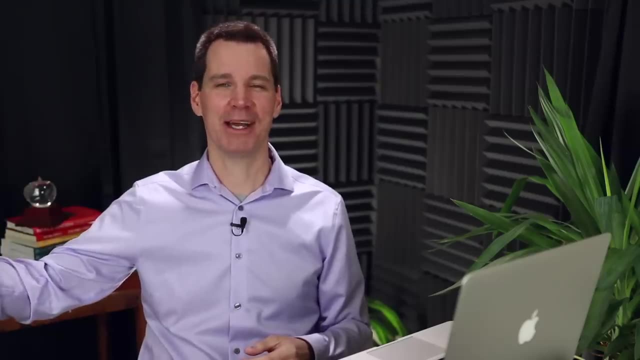 get up to use the bathroom or there'll be somebody with a lawnmower outside your window. In fact, I've been recording this morning and there's a neighbor working with a chainsaw nearby. that keeps distracting me, but you just power through it. So 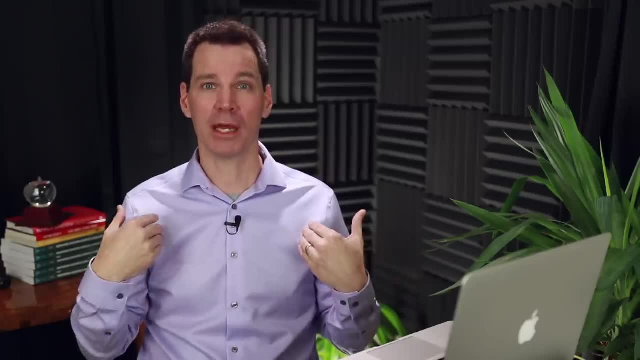 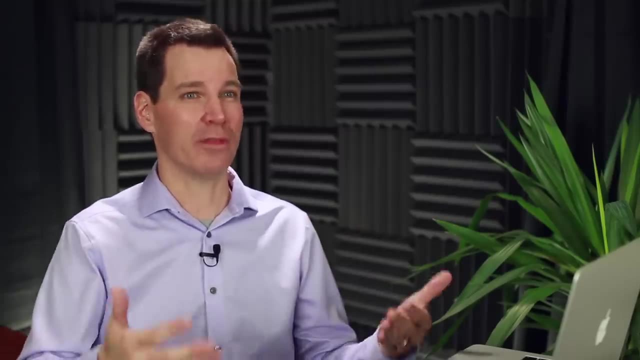 After a few times practicing alone. what I end up doing when I practice is I add distractions on purpose, Like I will put the television or some music on and then I'll talk over that, because it creates a little bit of noise and distraction for me to cope with And I know that. 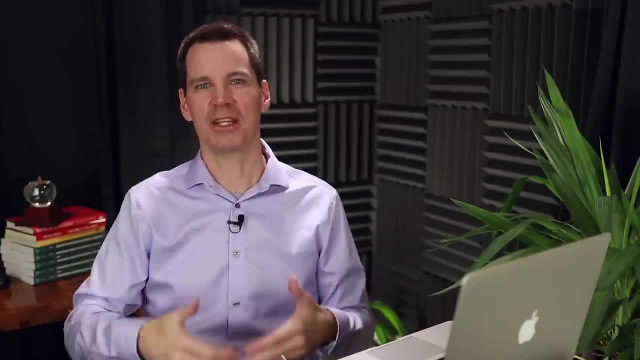 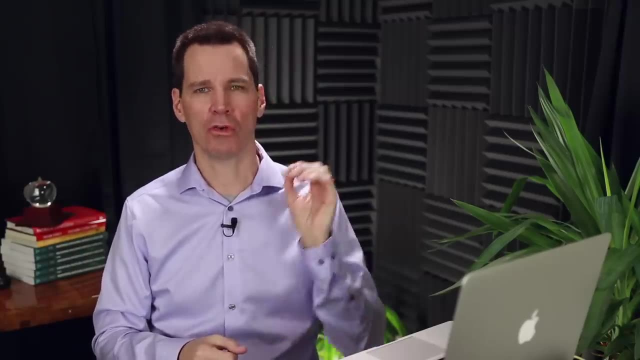 if I can practice through those distractions, that during the actual moment I'll be ready to push through, even if something weird or odd happens. it won't throw me off as much. So keep practice sessions realistic, And the number five tip is to visualize the first 30 seconds and the 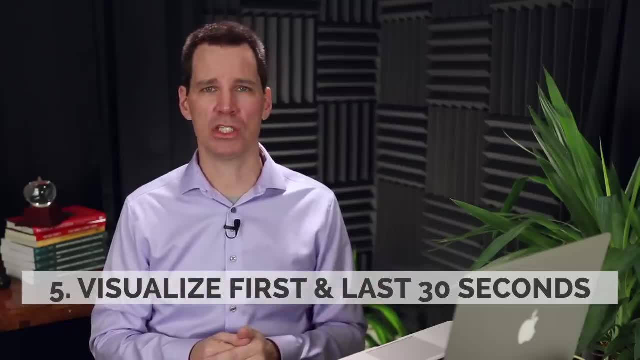 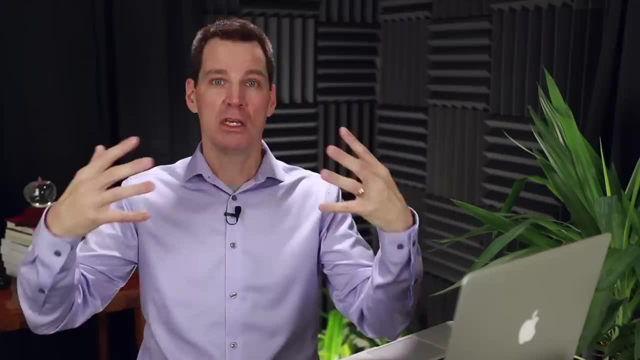 last 30 seconds of your presentation. So by visualization I mean the way a sports athlete does it. So you picture yourself walking up there that first 30 seconds of the moment starting off your presentation and then the last 30 seconds of how you're going to close. 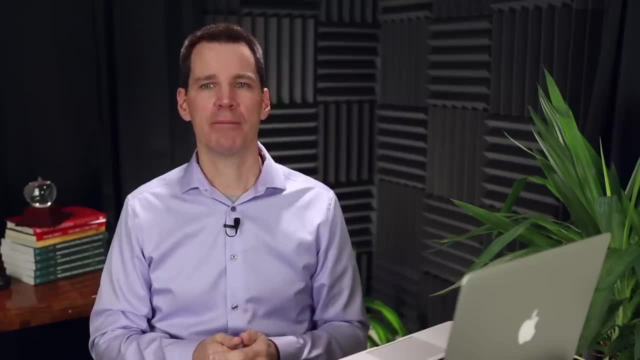 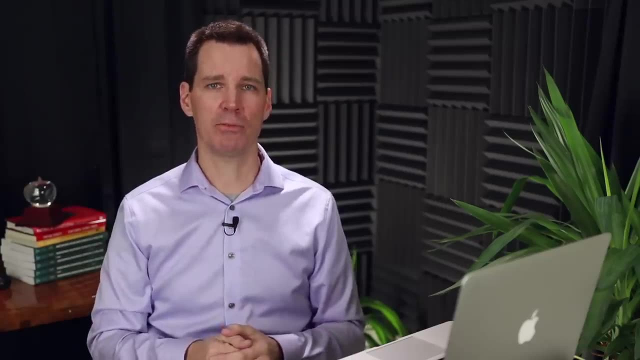 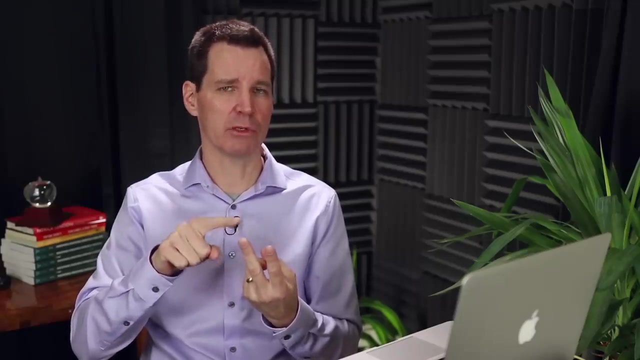 So athletes do this with great success. There was a study by Laurie Eckert published in the 1980s and a lot of other studies Like it on basketball free throw shooting And they found people that only visualized actually did improve a little bit. People who practiced free throws- basketball free throws improved a. 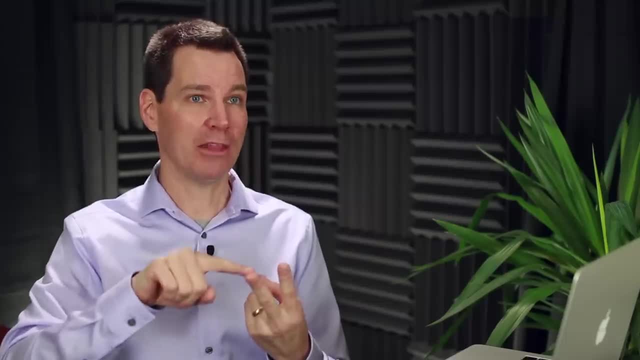 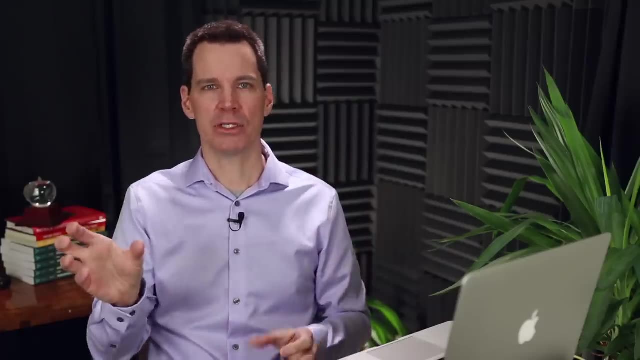 little more. But athletes who did both- they visualized and they practiced- did the most improvement out of any of the groups. So by visualizing their first 30 seconds and last 30 seconds, you're going to be boosting your overall performance up quite a bit, even if you don't get.